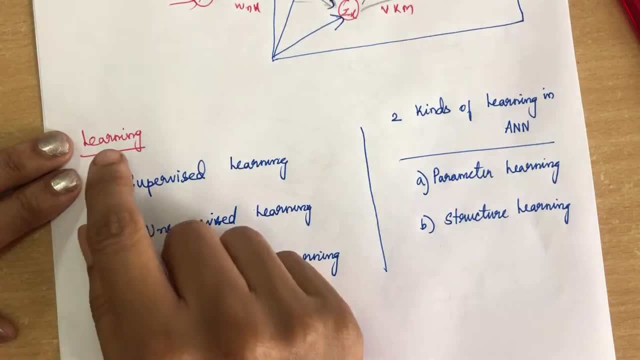 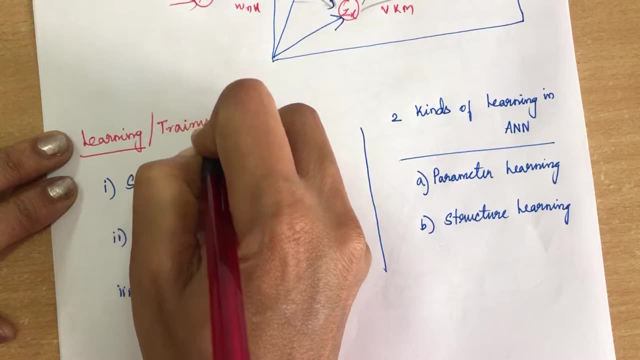 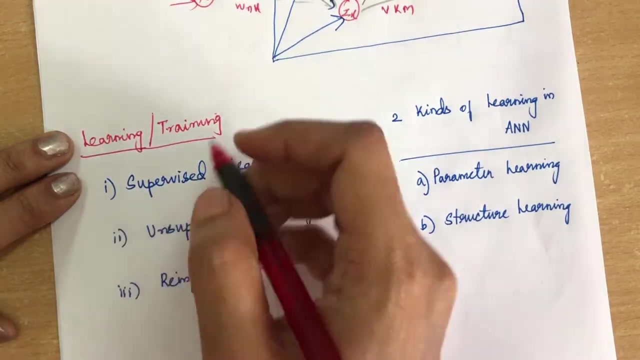 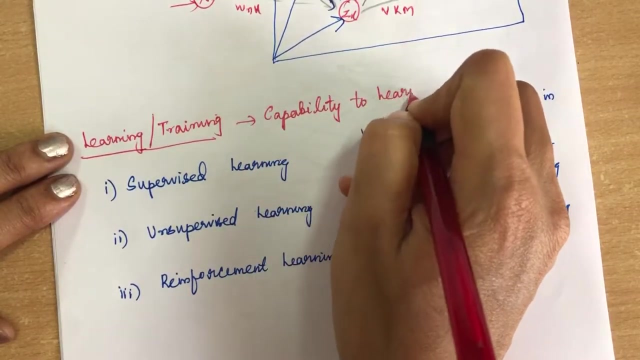 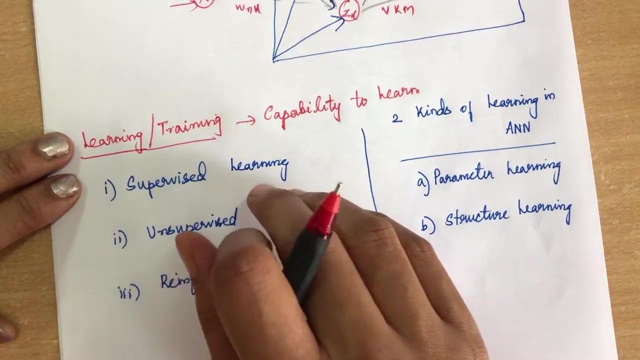 The second model in artificial neural network is learning or training. So what is learning or training? Learning or training in artificial neural network is adapt to itself or capability to learn. So the artificial neural networks has a capability to learn itself by looking its environment, or it has to change its own parameters such that it has to get the desired output. 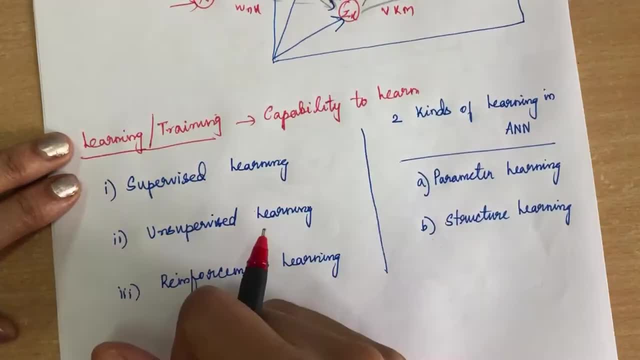 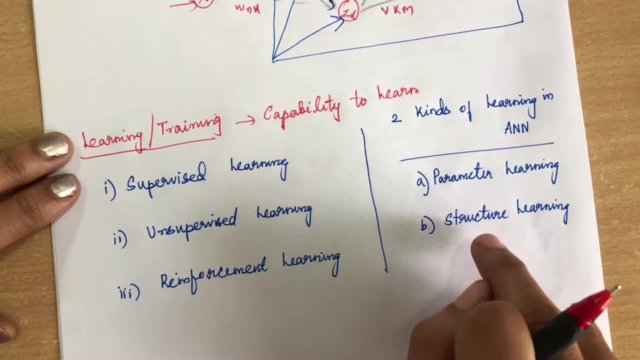 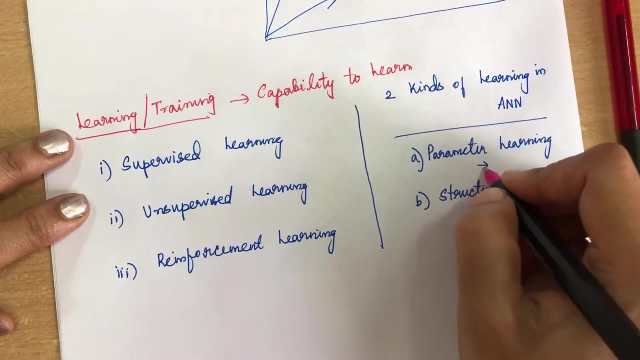 So to get the desired output it has to adjust its own parameters. Usually learning is done in ANN. There are two kinds of learning in ANN. One is parameter learning, other one is structure learning. What is parameter learning? Parameter learning means we will be adjusting the weights. 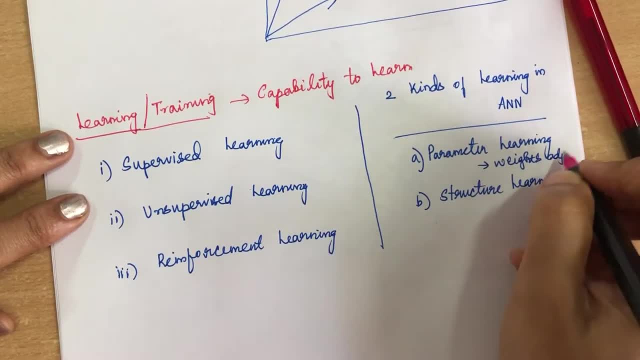 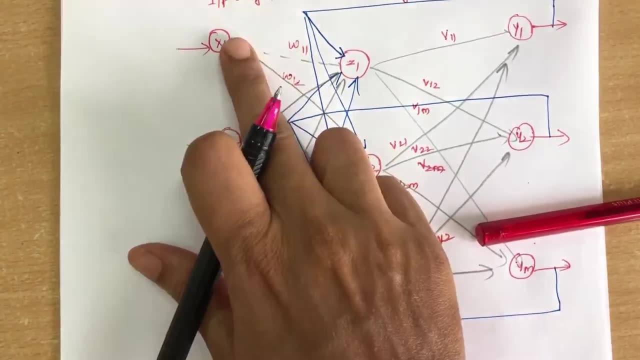 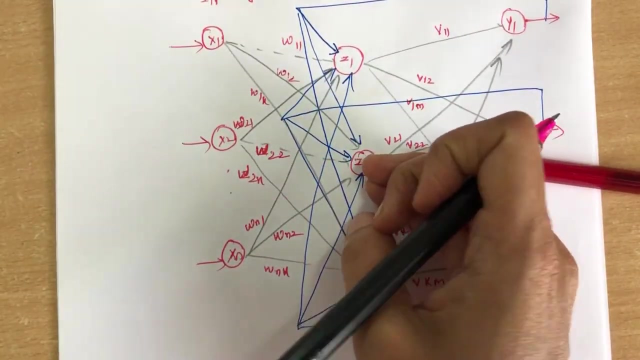 weights. adjusting weights will be adjusted. That means here, as we all know, we are assigning initial weights. We are assigning some weights over here to the network between the nodes. So these weights are initially will be assigned between the value 0 and 1.. So when you are training the network, these weights will be adjusted so that we will. 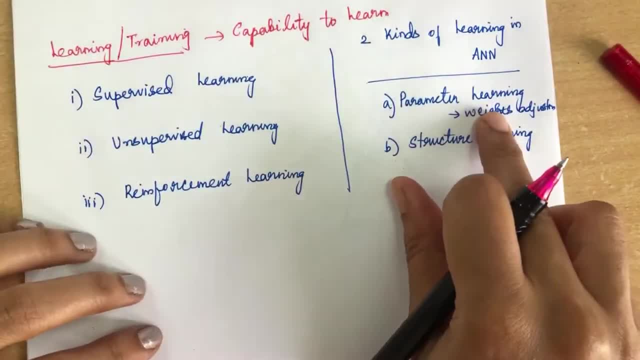 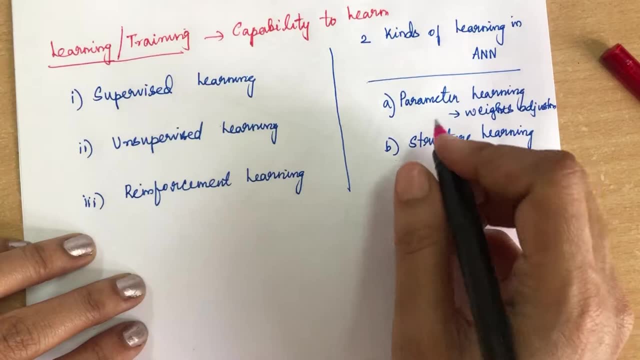 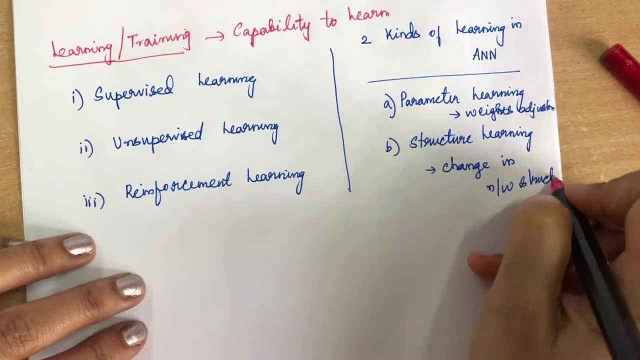 get the desired output. That is called as parameter learning. That means you are going to adjust the weights between the nodes. What is structure learning? Structure learning means it is a change in the network structure itself. So that means you can change the number of 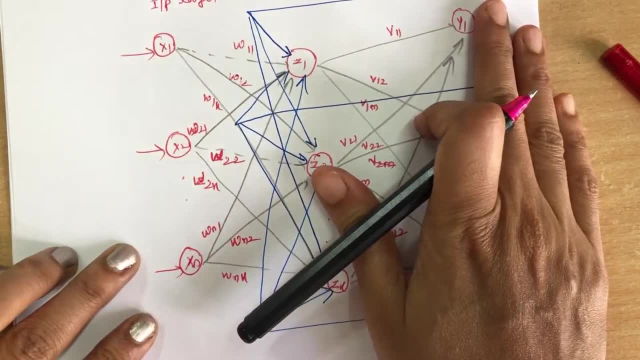 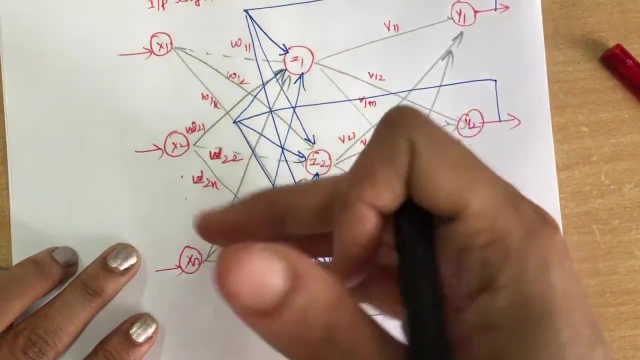 suppose you are going to learn this particular. initially you have given this type of network. Now, when you are going to learn this network, you will be changing some elements. Suppose you will be removing this processing element, you will be adding some more processing element. So there, 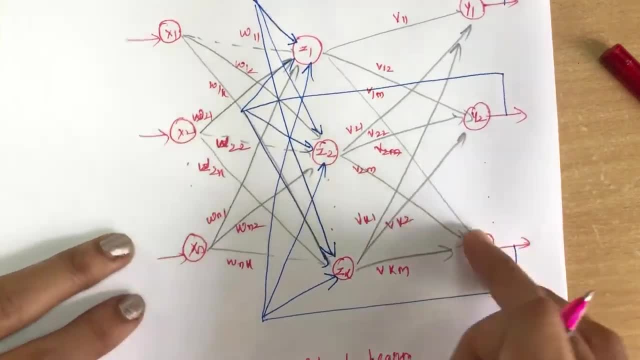 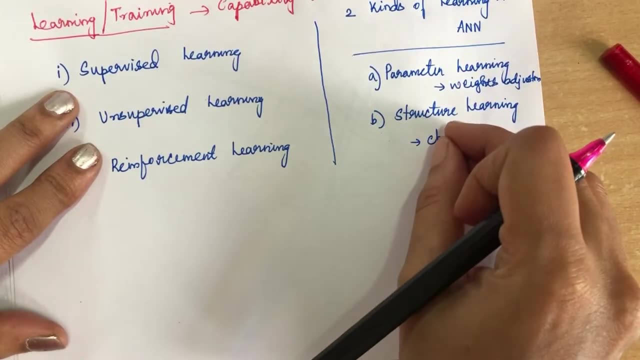 will be change in the network topology itself. That is one type of learning. So second learning is structure learning, and first learning is parameter learning, where we will adjust weights. Okay, these are all two kinds of learning, And apart from these two kinds of 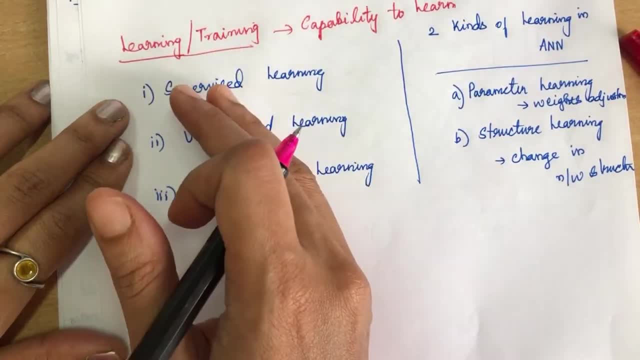 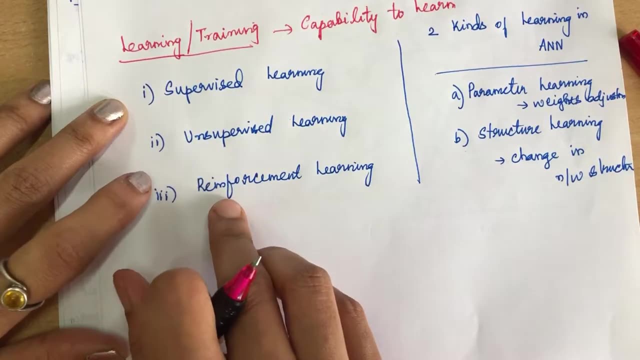 learning you have in ANN. it is again it is broadly classified into. learning is broadly classified into three types. One is supervised learning, unsupervised learning and reinforcement learning. We will see one by one now. Now we will see about supervised learning In supervised 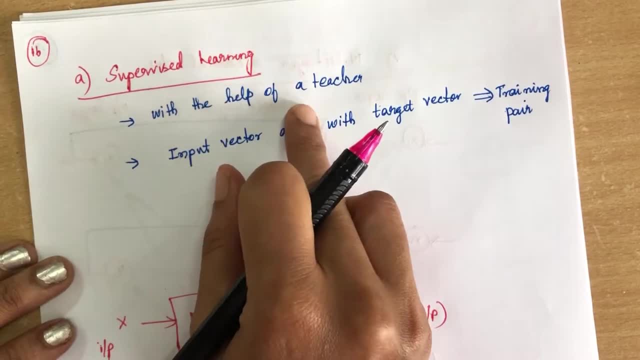 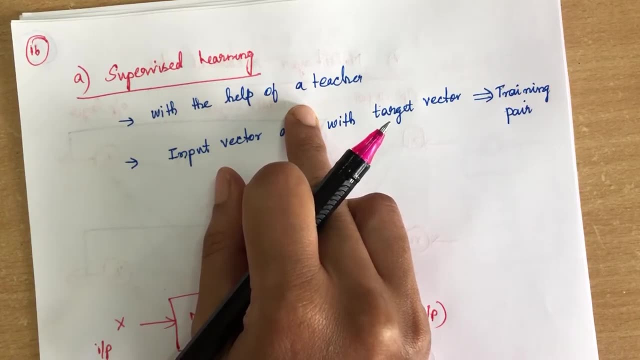 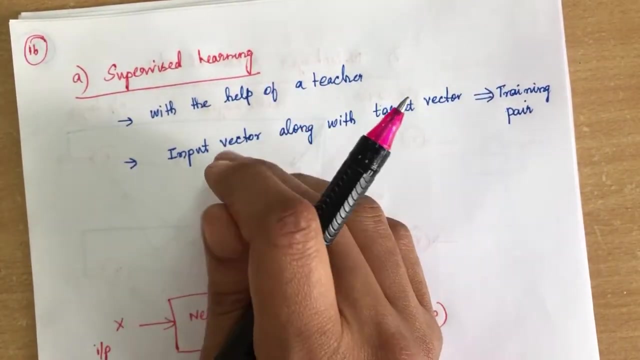 learning. learning is performed with the help of a teacher. Now I will explain with the help of a example. let us take an example of a small child. so when the child is in home, the mother teaches everything. when the child goes to the school, there will be a teacher to monitor him, so the teacher helps him. 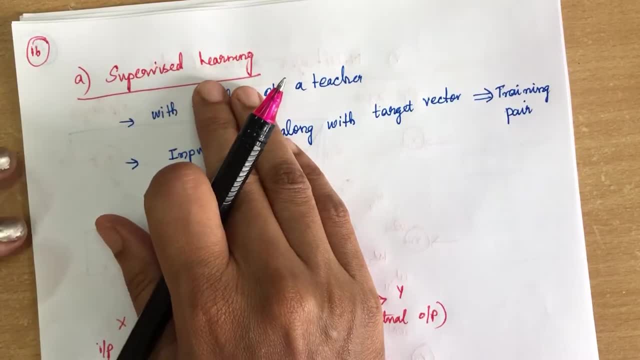 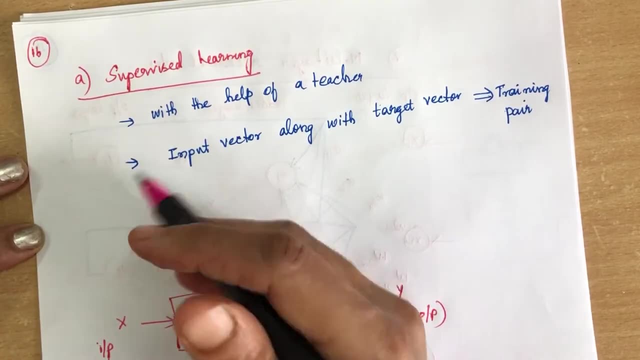 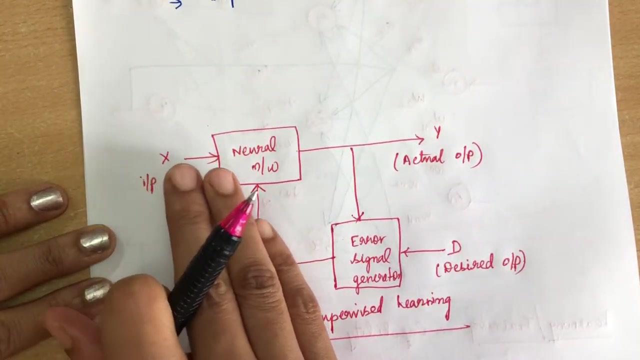 in his studies. so this type of learning is called a supervised learning. so this: we will see how this ANN uses this type of concept, so here in supervised learning. so, for example, we will take this diagram: this is supervised learning. you consider that there will be. you will be given an input values. 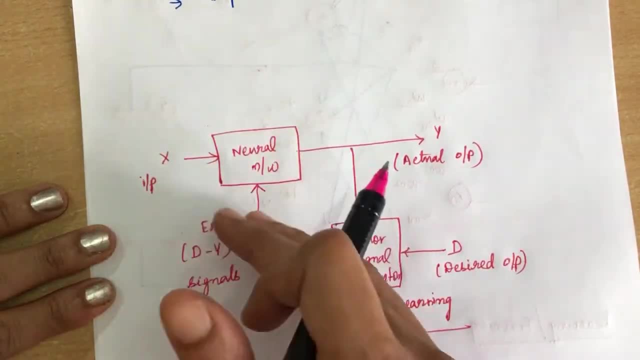 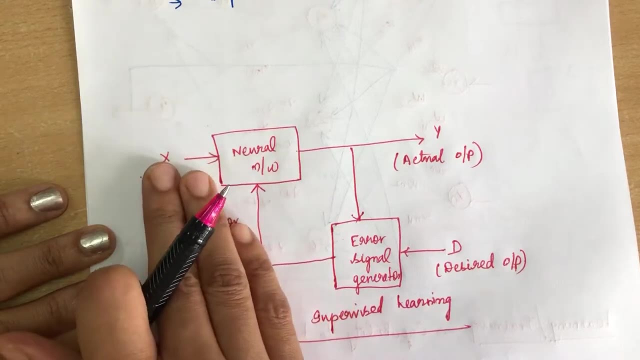 to the neural network. here I have not drawn, I have not given drawn all the nodes. simply I am giving the neural network alone. you can use any type of network topology, so the input nodes, the input values will be given to this neural network. it will give you some output, right? so how do you? 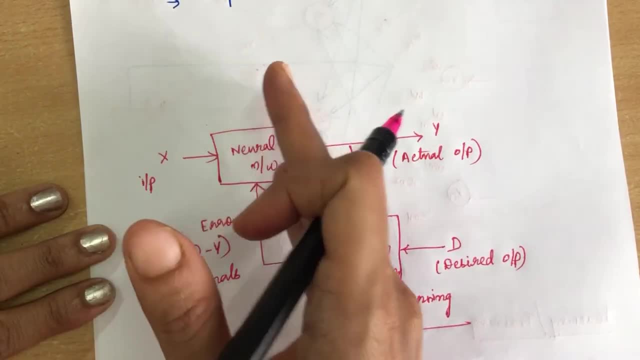 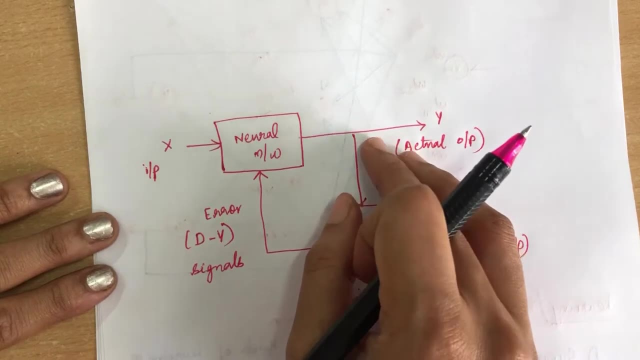 calculate the output. you will be multiplying the input values with the weight values and you will get the output, some output you will get. this is your actual output. so now what we will do is this output. it will be compared with the desired output. what is desired output? so desired output is nothing. 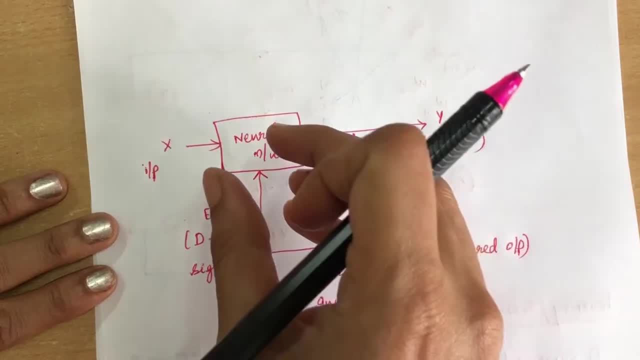 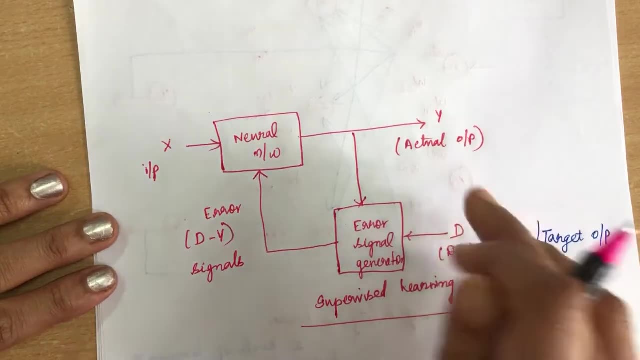 but then this is your target output. so your network should achieve this target output, desired output or otherwise called target output. okay, this is output you have got, with help of this, weight values and input values, but you have to compare it with the target output. so now the supervisor what will do? is it now they will compare your actual output with the target? 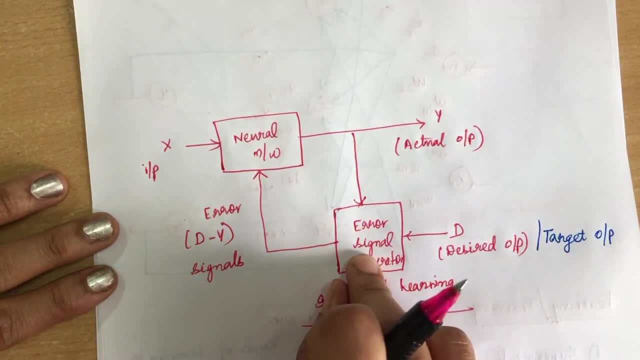 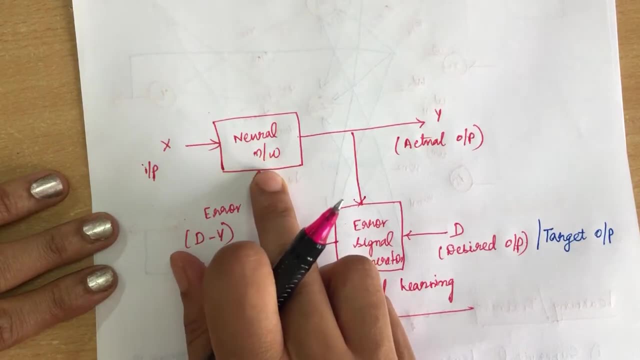 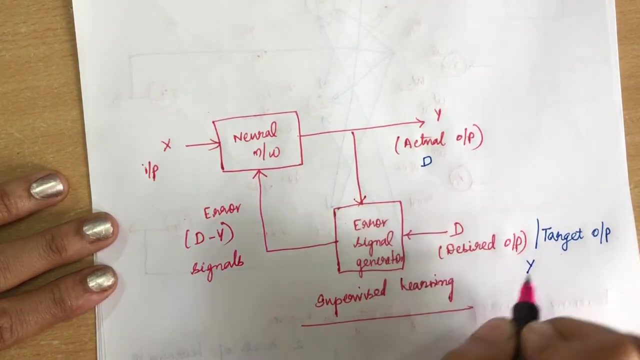 output and it will generate an error. if any error is there between actual output and target output, that will be given as a feedback, that is, it will be given as an feedback to the neural network. so here what happens is this. we can call it as: actual output is d and target output is y, and we 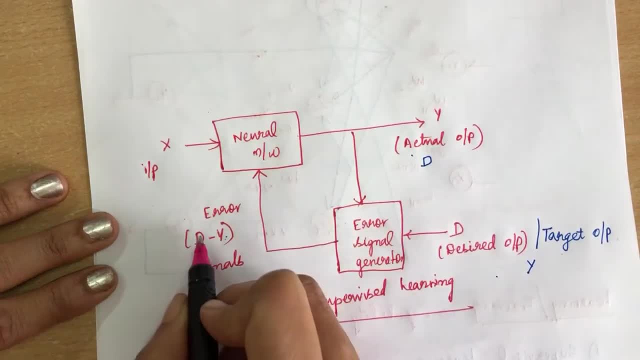 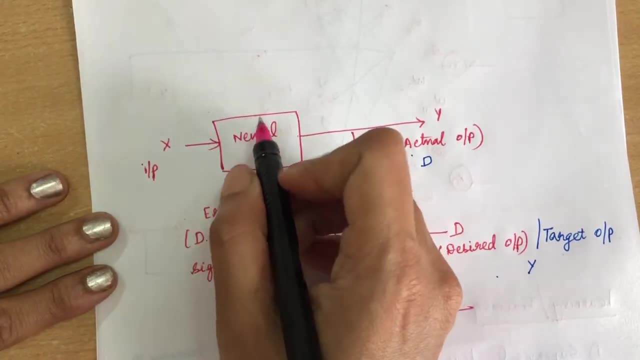 will find out the error by subtracting d minus y, that is, d minus y. this error will be given to this neural network. using this error, we what we will do is we will adjust the weights again, we will calculate the network. so how we will calculate? we will multiply that, we will take. 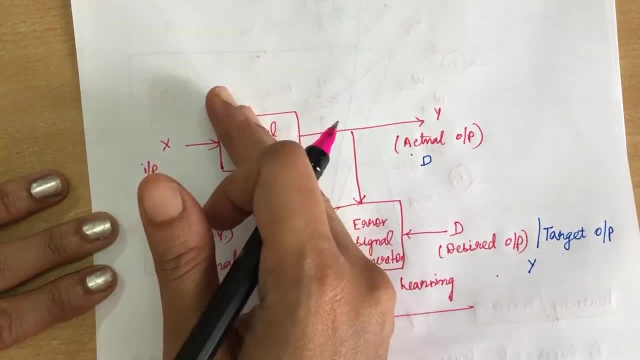 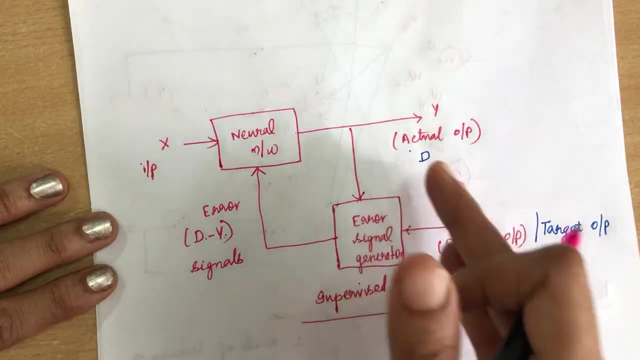 the summation of multiplication between the input values and the new weight values. again we will find out the actual output. so this actual output is again compared with target output and we will find out any error. is that if the actual output closely matches? if it matches, we will repeat this. 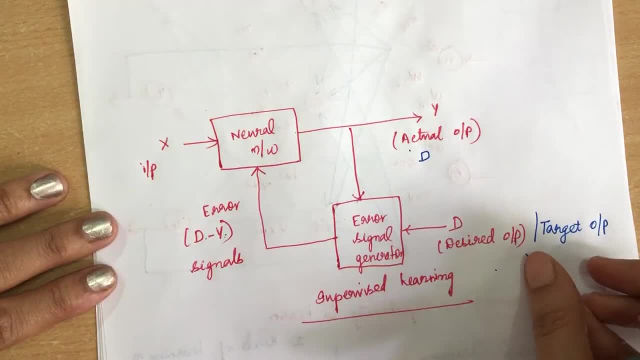 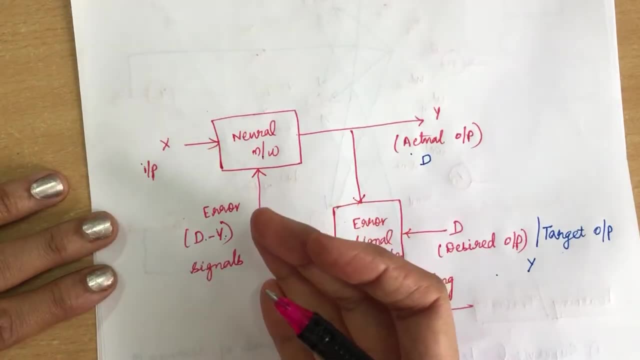 work until this actual output closely matches with your target output. when it matches, we will stop training. this is called training. so what do you mean by training over here? training over here is nothing, but suppose, for example, if a teacher wants to, if suppose if the teacher is teaching the child. 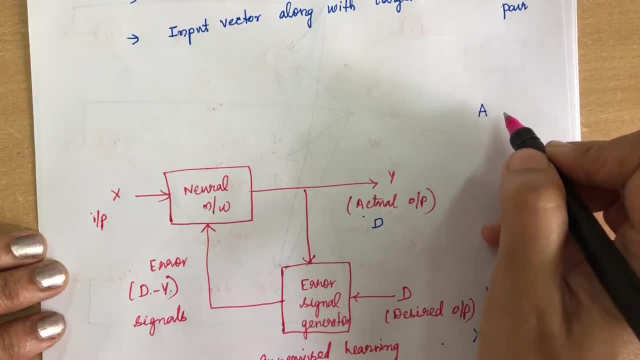 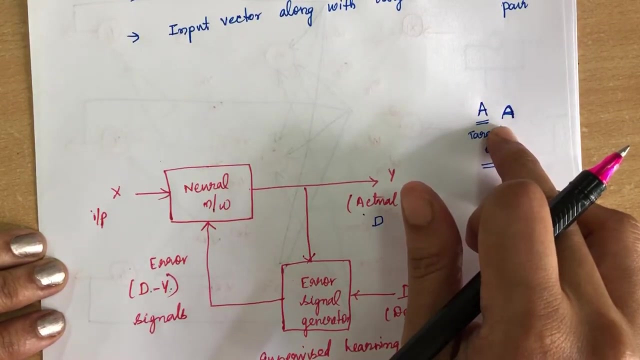 to get to the alphabets. okay. so the student, the child, is writing like this instead of lighting. like this is my target output. right, this is my target output. i have to achieve like this, but the child is writing like this. so what the child teacher has to do, he has to help him. so 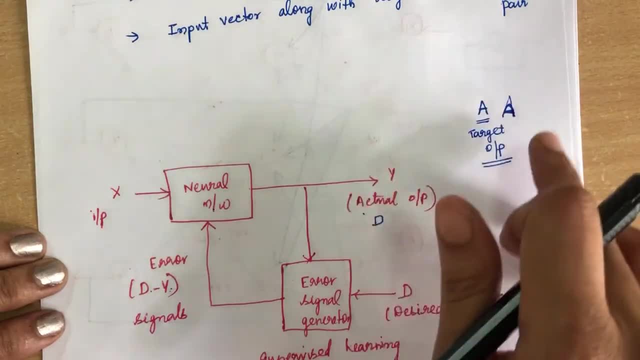 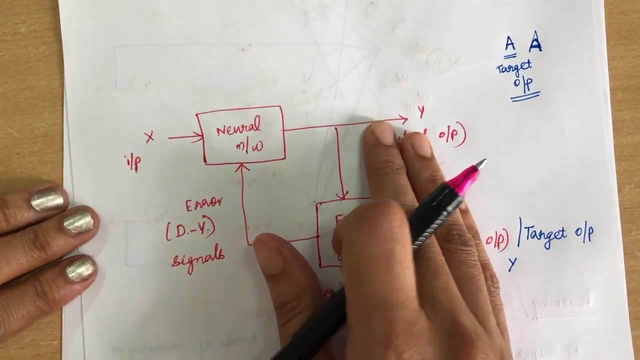 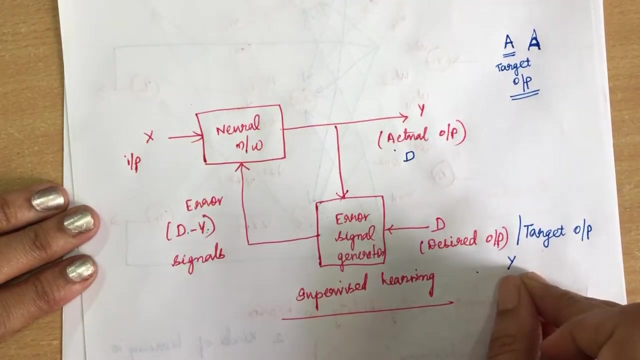 that he will get the desired output. this is called as training or learning. so this is what we are going to do: it in neural network also. so we are going to find out that some output using this network, we are going to find out the actual output and we using this and we are going to compare it with the target output. 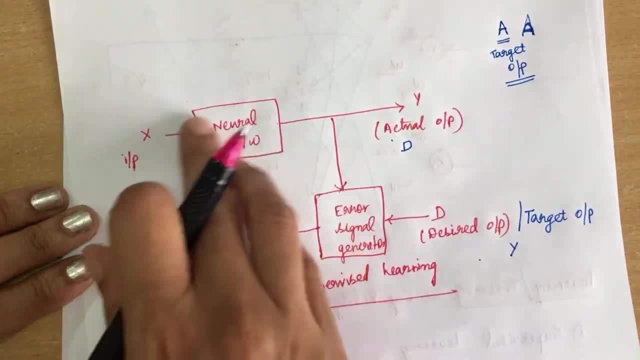 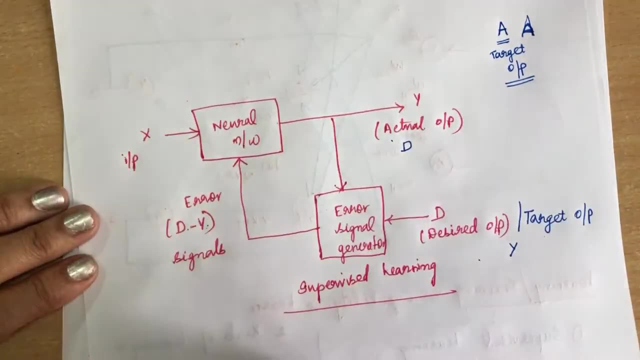 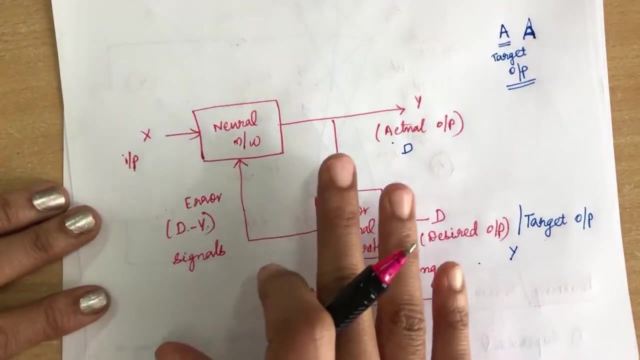 and if there is any difference, again we will be doing some modifications and we will get the output. so again we will be doing this. this procedure will be repeated until the actual output matches with your target output. this type of learning is called as supervised learning, so we will say that the input vector 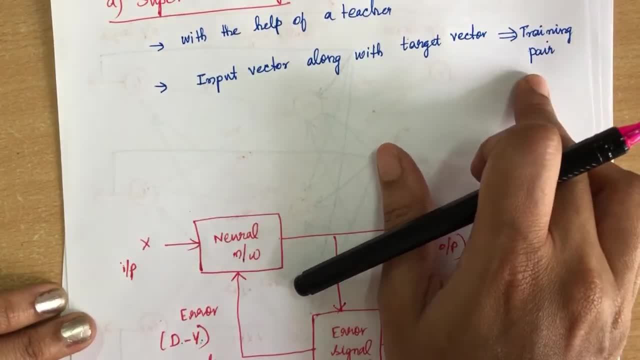 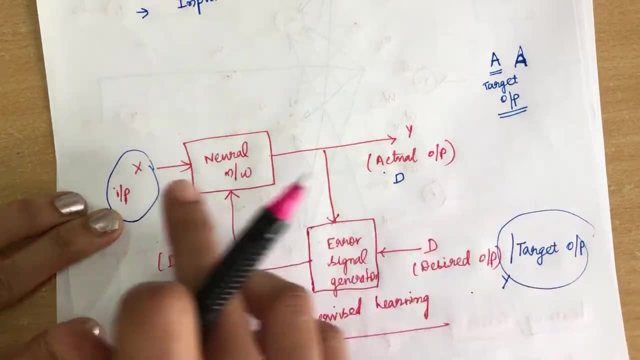 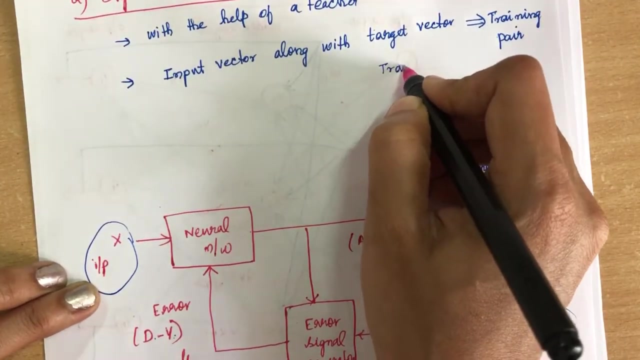 along with target vector, is called as training pair. so the input values know this: input values along with the target value. you call these this pair as your target training pair. this pair, you can call it as a training pair. so training pair, what do you mean by training pair? training pair is nothing, but it consists. 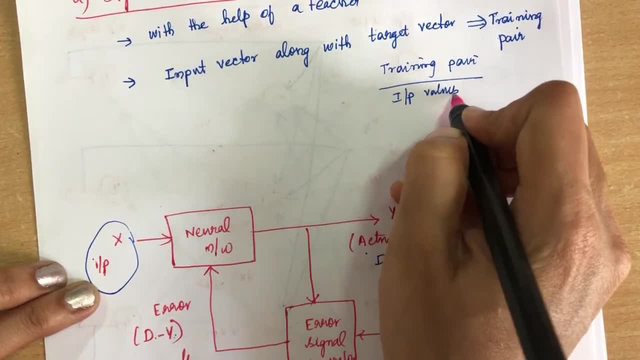 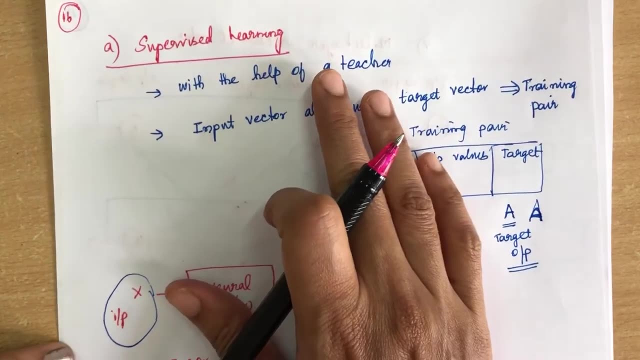 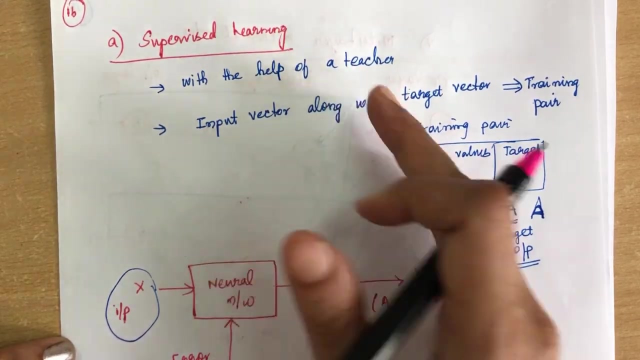 of input values and training values, the target values. so this is called as training path. so in supervised learning you will be, it will be, you will be training the network with help of a teacher. okay, so how teacher monitors the child. likewise we are going to monitor, we are going to monitor this network by learning. 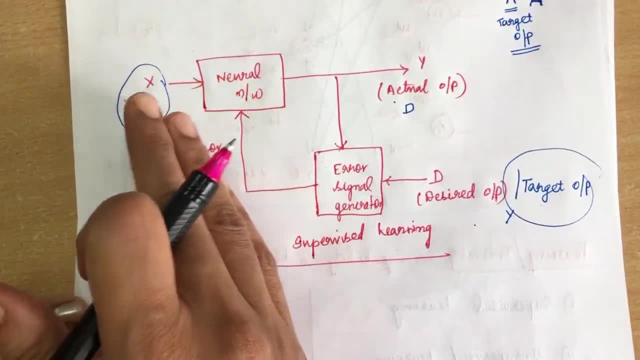 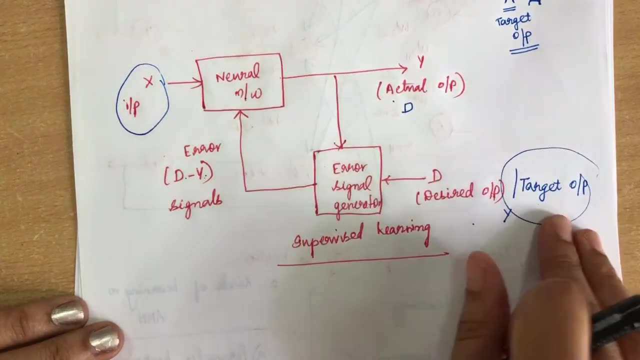 so by training or learning so how it does. so we are going to present the input values to the network and weight values will be there. according to that, we will find the actual output and this actual output is compared with target output and we will train the network by giving as an error. and again, 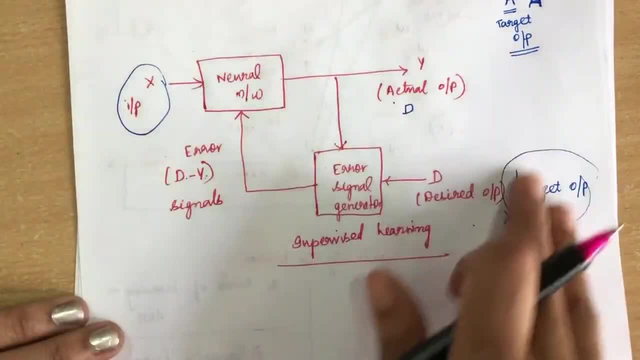 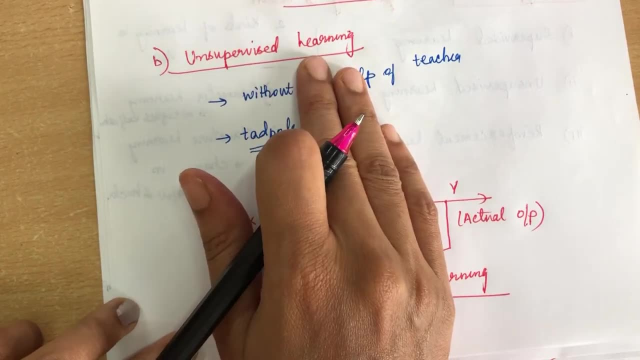 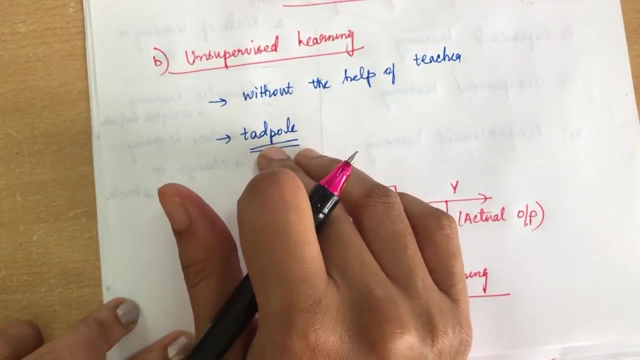 we will adjust the weight values again. we will find out actual output. this procedure will be repeated until we will get both the values matches okay. second learning is unsupervised learning. in unsupervised learning, the learning is performed without the help of a teacher. let us take an example of a tadpole. so tadpole, when it is born, it is there, is nobody, is there. 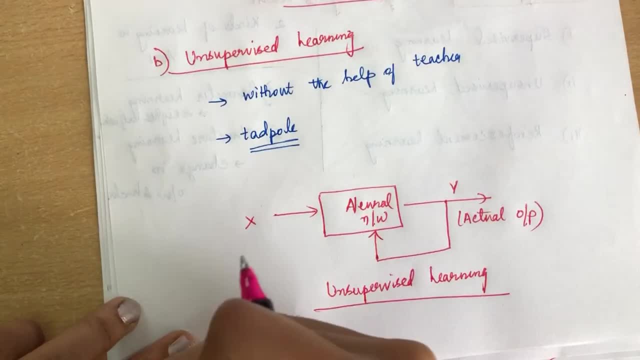 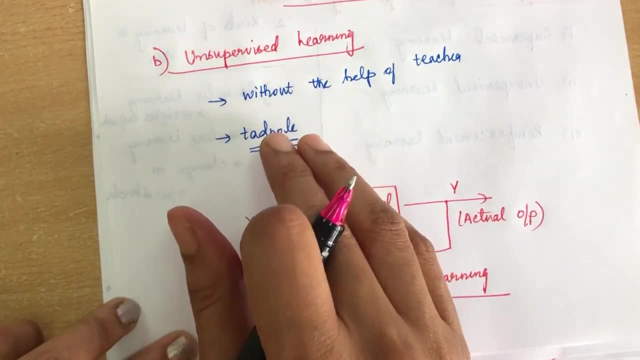 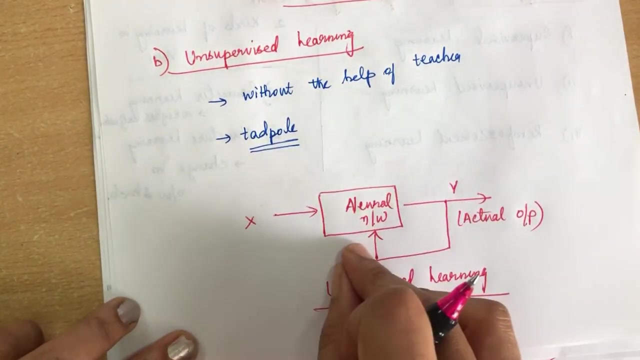 to teach how to swim. it learns by itself. so here it is. this process is independent and there is no supervisor or teacher to monitor him how to swim, so it learns by itself. so we are going to achieve this concept in unsupervised learning, like in neural network. so here, if you can see this, here we don't have a target output. 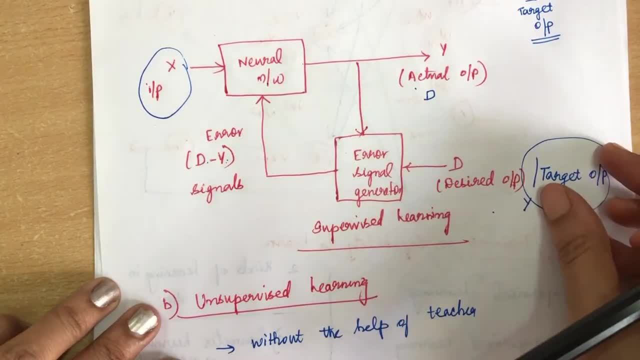 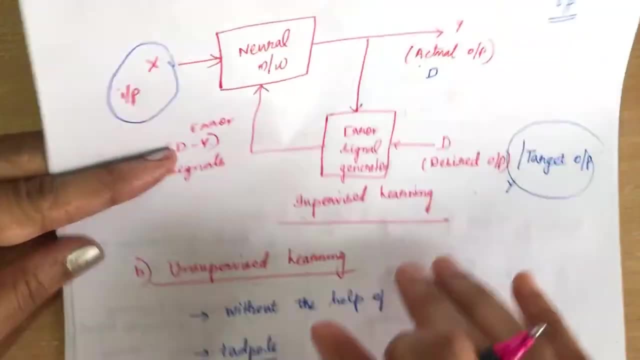 see here. in case of supervised learning, we have a target output. this is your target, so we can achieve this target by giving this error as an feedback to this neural network. but coming to unsupervised learning, since there is no target values, the input values will be sent to neural 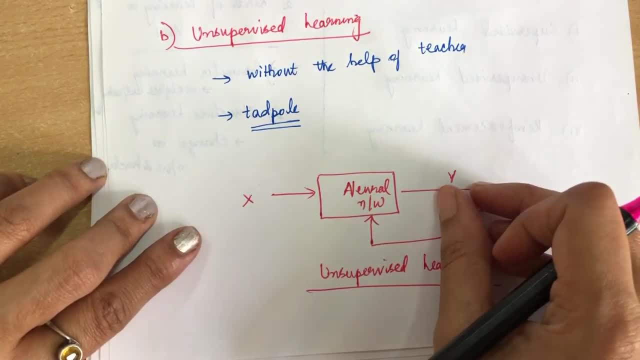 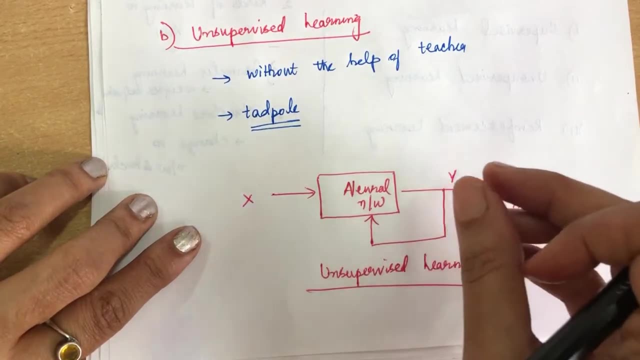 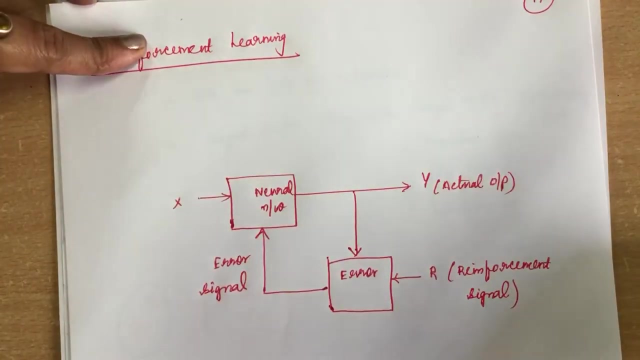 network. it will produce output. so this output values. we doesn't know whether this output values correct or not. there is no supervisor. is that to tell whether this output values is correct or not? this type of learning is called as unsupervised learning. third learning is reinforcement learning. 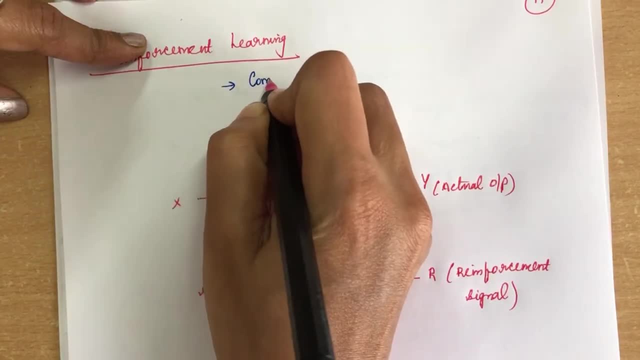 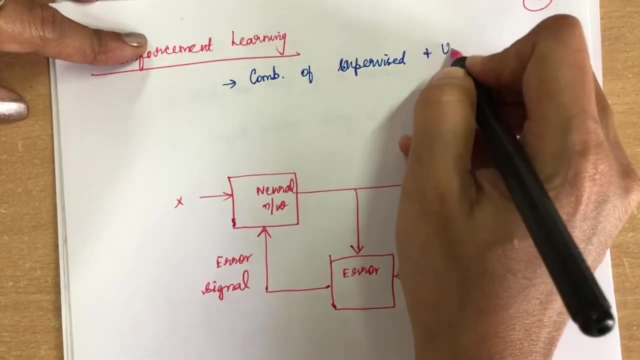 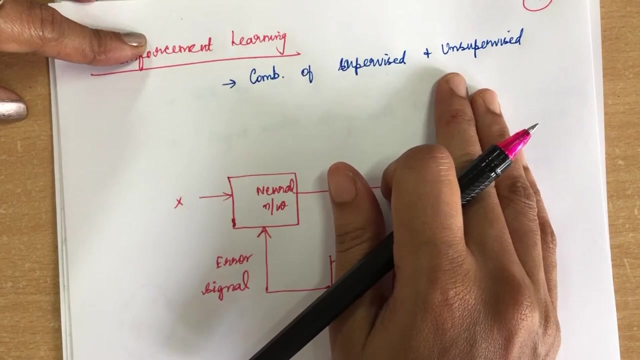 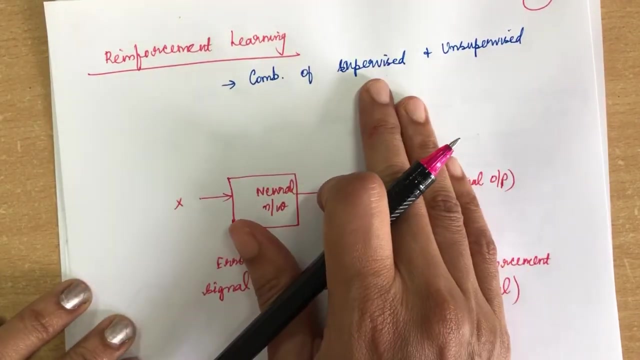 reinforcement learning. it is a combination of supervised learning and unsupervised learning. supervised and and unsupervised. so what is supervised learning? there will be a teacher to help, but an unsupervised. it is an independent process. there will not be any teacher. so this reinforcement learning, it is a combination of both. so in supervised learning, what we will do is 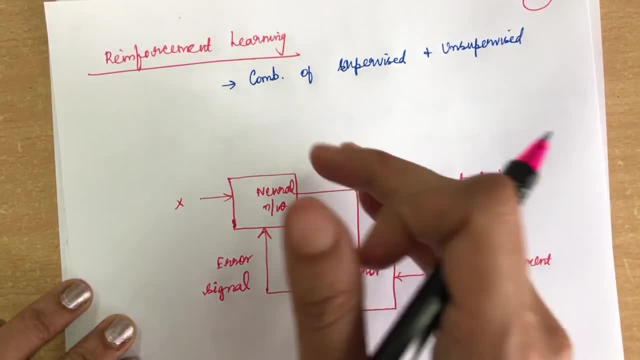 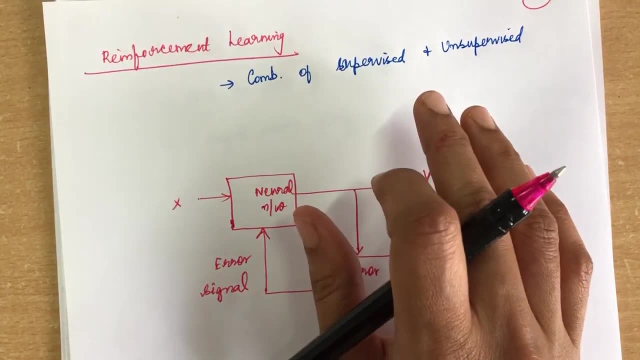 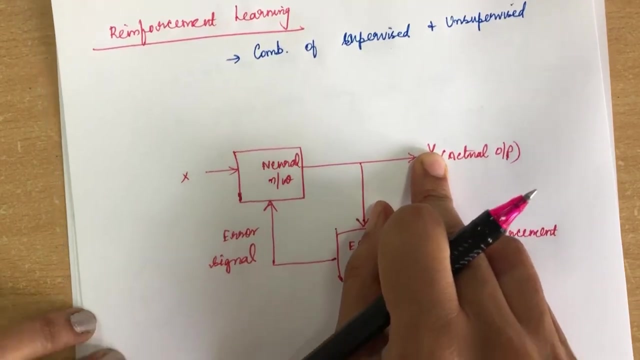 we will be presenting the actual output itself. but in case of reinforcement learning, we will not give the actual output, but only less information will be given. you will see how this reinforcement learning is used in neural network. so here, x input values is given to neural network and you will get some actual output. this output it will be, you will be. 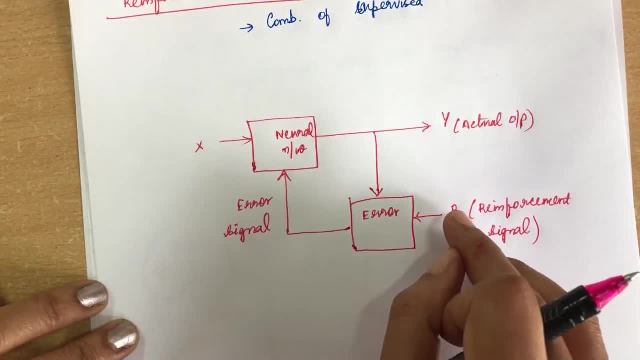 given less information that is like actual the target values will not be given. it will be only critic information will be given. that is like the teacher will be given only critic information. what he mean by critic information, that means he will say whether the actual output is correct or not. 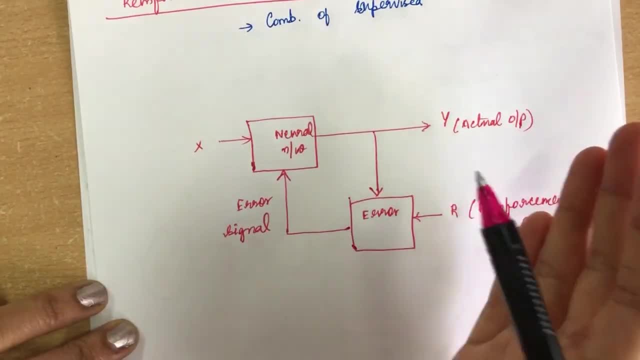 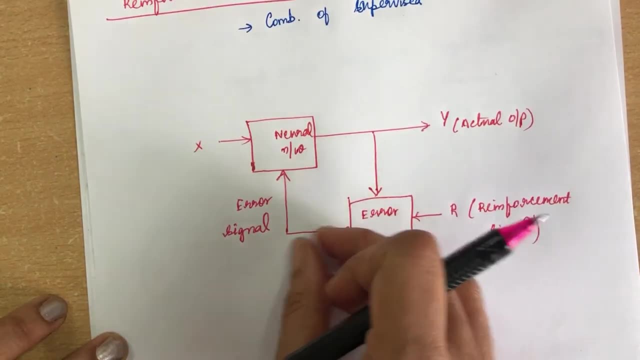 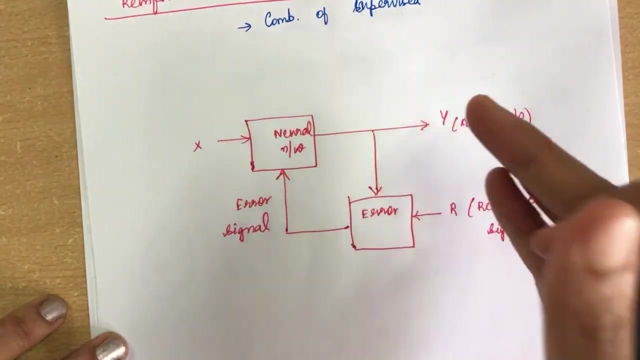 he will give you only 50 percent result. it let us. it will say that whether the actual output is correct or not, based on this error should be generated, and this error will be given to the neural network. and then again it has to adjust the network and it has to press, it has to get the new output, it has to ask for the teacher. 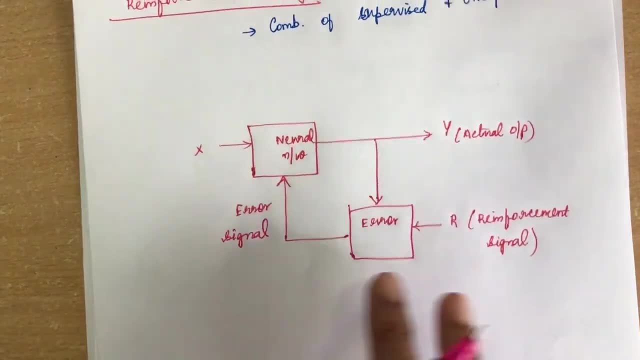 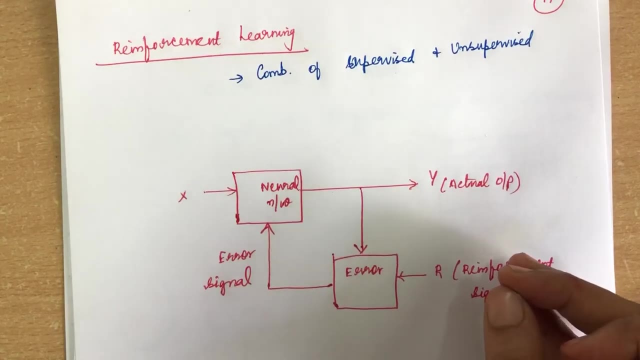 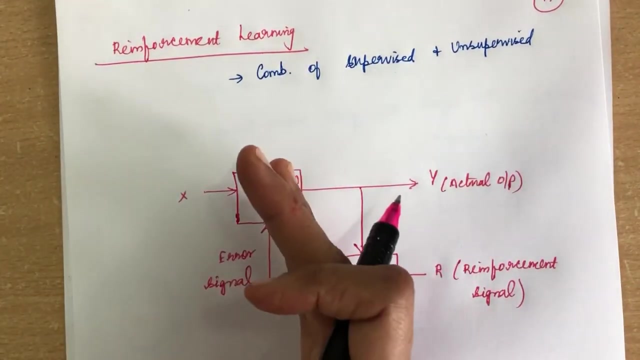 so he will tell whether it is output is correct or not. so this type of learning is called reinforcement learning. so we don't, the supervisor will not give you the exact target values, but here the supervisor will tell you that output is correct or not. this type of learning is called as reinforcement learning. 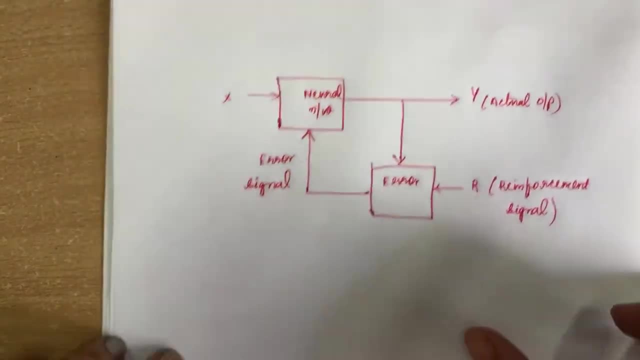 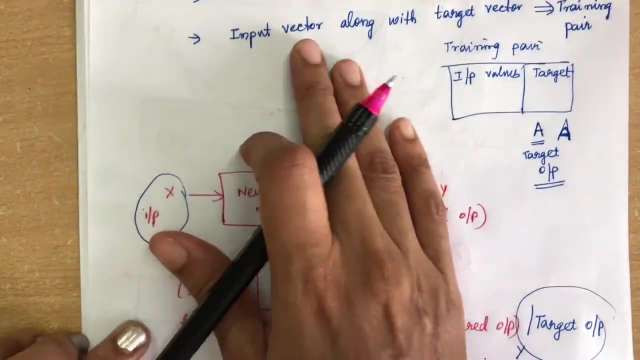 so in this we have learned three types of learning. one is supervised learning, second one is unsupervised learning and third one is reinforcement learning. in supervised learning we will- we will have a teacher to help, so like, for example, we will, we'll be given the target. this is the target values we 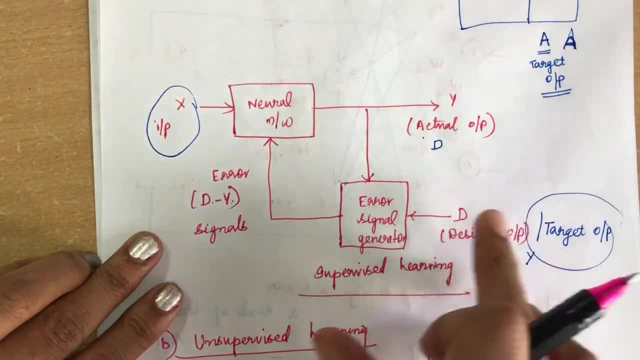 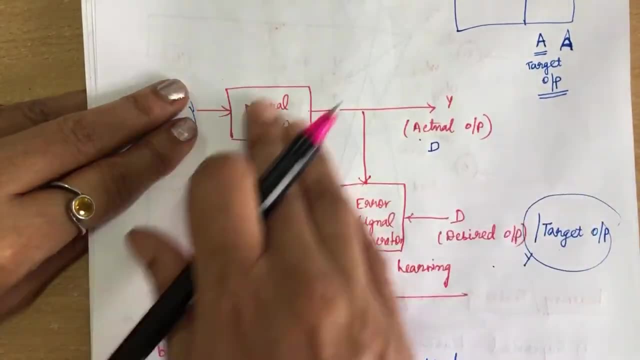 will know. so we will compare the actual output with the target values and, using this, we will find out the error and we will ask them to adjust it and we will get the new output values. and this type of procedure is called supervised learning. coming to unsupervised learning, there will not be any teacher. 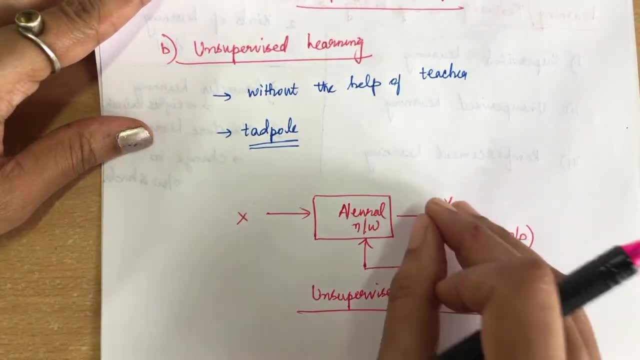 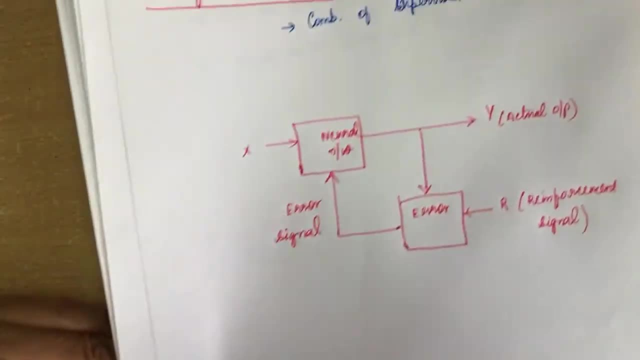 so just, we have to produce the output, but we doesn't know whether the output is correct or not. so, based on our assumption, we have to get the output. this is unsupervised learning. third one is reinforcement learning, where it is a combination of both supervised and unsupervised. so here the 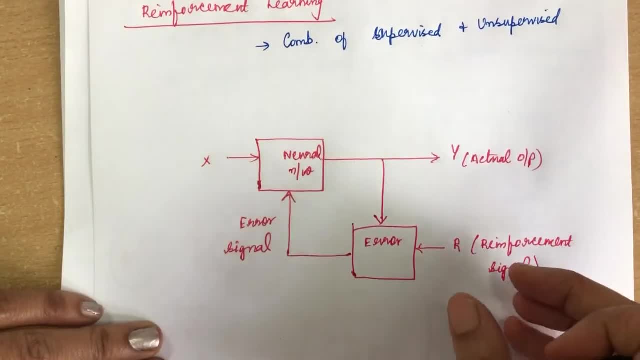 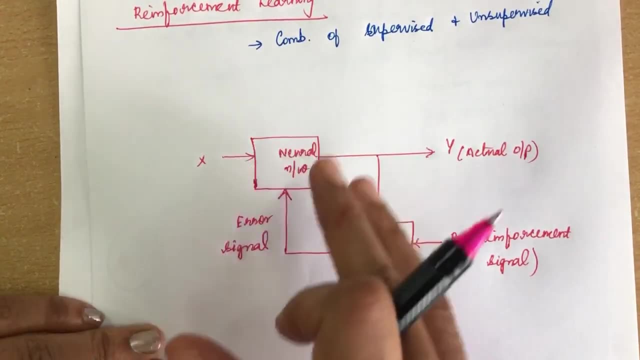 teacher will not tell the exact output. he will give you the. he will tell that, whether the output is correct or not, based on that, the error will be generated and this will be given as an input to the neural network to adjust the weights and they will present. 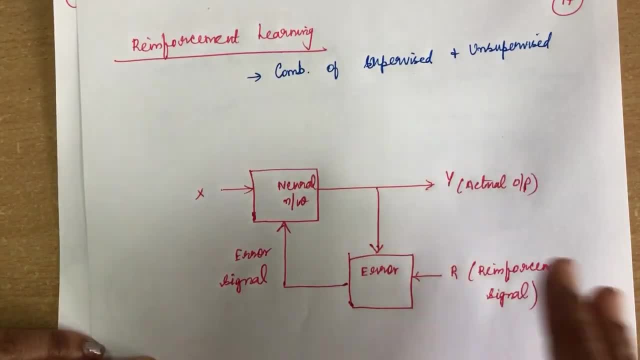 it will give you the new output. likewise, this, all these learning is. these are all three- three types of learning in neural networks.